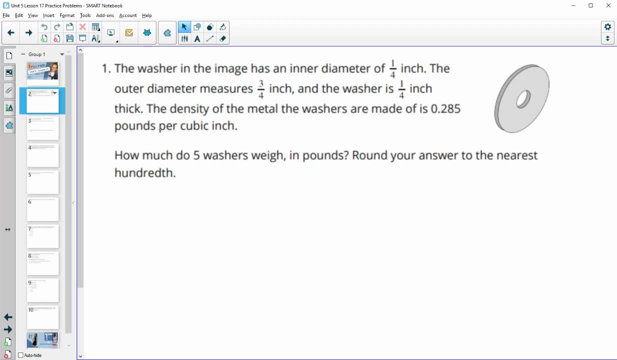 density of the metal is 0.285 pounds per cubic inch. We have five washers and we want to know how much they weigh, So remember that. you learned that the density equals the volume divided, or sorry, the mass divided by the volume, And so we're looking for the mass in this case, So we could. 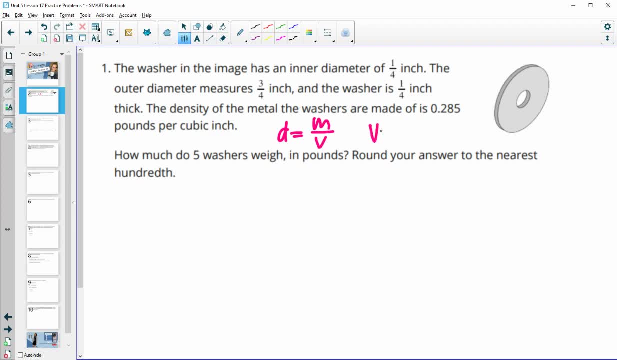 just multiply v to both sides. So really we're going to be doing the volume times the density and that's going to give us the mass. So we want to find the actual volume of this washer. So this washer is like a cylinder, just. 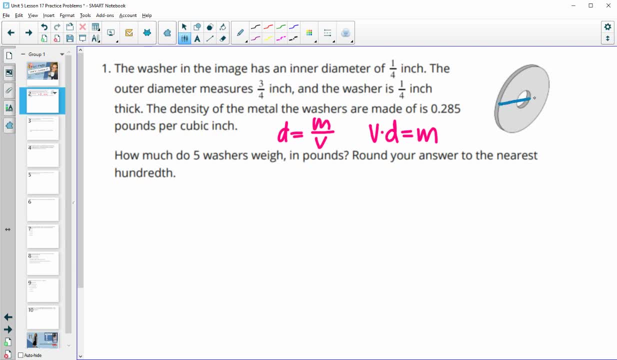 with a cylinder missing in the middle. So remember that the diameter all the way across here was three quarters of an inch. And so if we found the radius, so if the diameter is three fourths of an inch, then the radius is going to be half of that which is going to be. 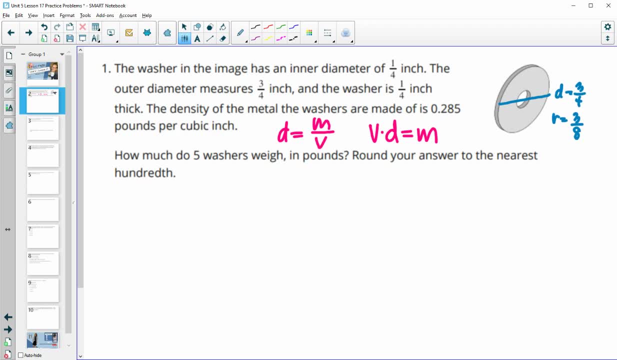 three-eighths of an inch, And you can certainly do that in decimal form. So you could do 0.75 divided by two and get your radius for that larger circle or for the outer part to be 0.375.. So then we're going to want to find the area of that, And the area formula is pi times the. 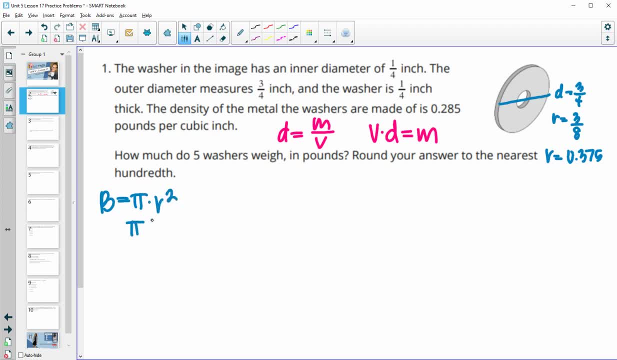 radius squared. So we're going to do pi times the 0.375 squared, And then you're trying to do volume. So remember, volume is area of the base times the height. So we're then just going to multiply this by the height of the cylinder And the height of the 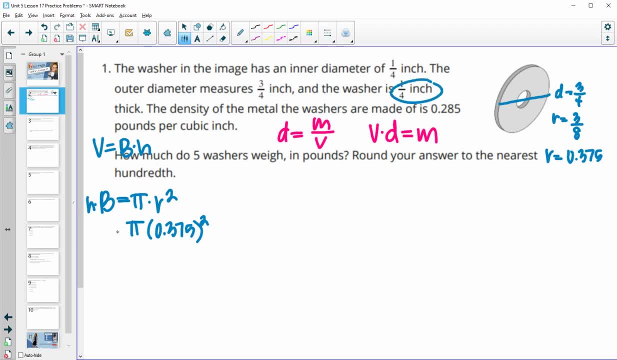 cylinder or the thickness of this washer is a quarter of an inch. So then we'll multiply this by 0.25 to get our volume. And then we're going to multiply this by the height of the cylinder, So we're doing area of the base times that height, So then the volume filled in, So the volume of 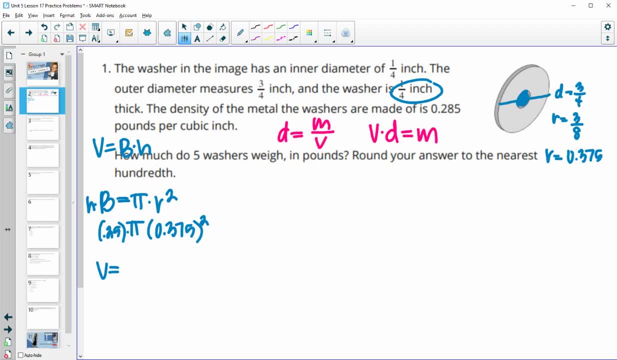 this whole cylinder right here is going to be 0.25 times pi times 0.375 squared, And that's going to give us a volume of 0.1104466.. So I'll just put to four decimal. so that's if we had just a filled in washer. Okay, so just a whole thing, no hole in the middle. 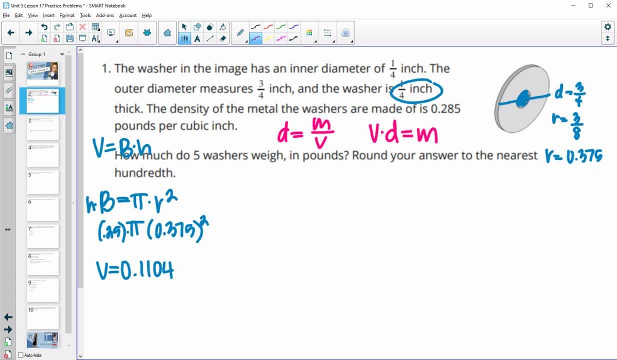 So then we want to find the volume of this piece that we're taking out. So the radius or the diameter here was 0.25.. And so again, we'll divide this by two to get the radius of that inner part, And that's going to be 0.125.. 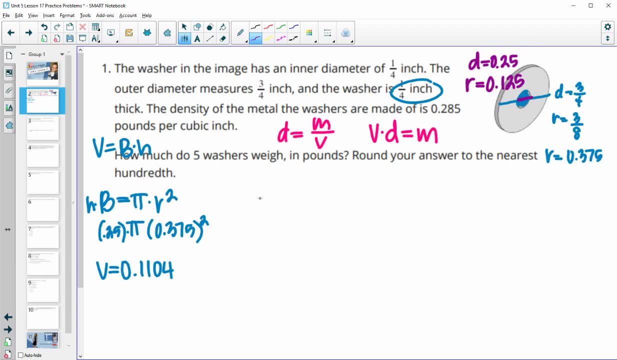 So we'll go ahead and find the volume of that cylinder. Okay, again, first finding the area of the base, And the area of your base is pi times your radius, 0.125 squared, And then the height of this or the thickness of the washer is still 0.25.. So we'll multiply this out And that will. 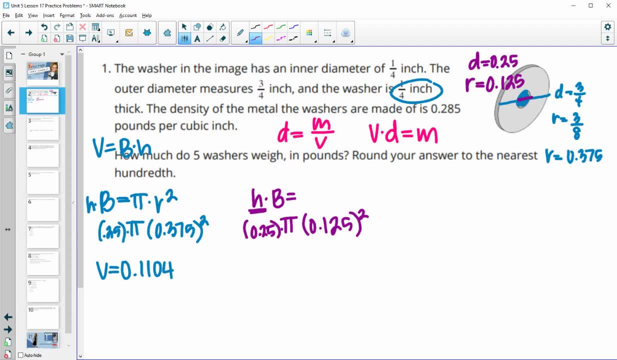 give us a volume. So that's going to give us a volume of 0.0123 for that inner part. So then the total volume of our cylinder or of our washer, So the volume of the washer you need to subtract these. 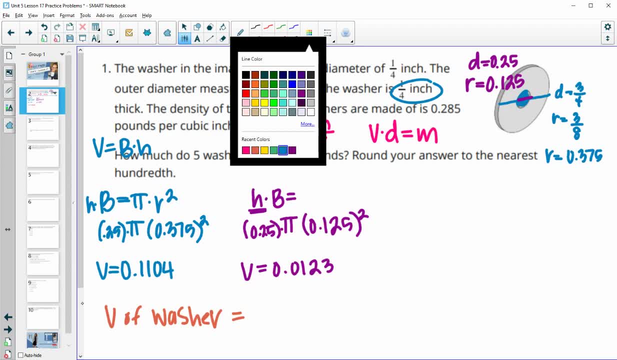 So we need to take that blue number here. So this one is as if it was filled in, And then we need to subtract these. So we need to take that blue number here. So this one is as if it was filled in, And then we need to subtract these. 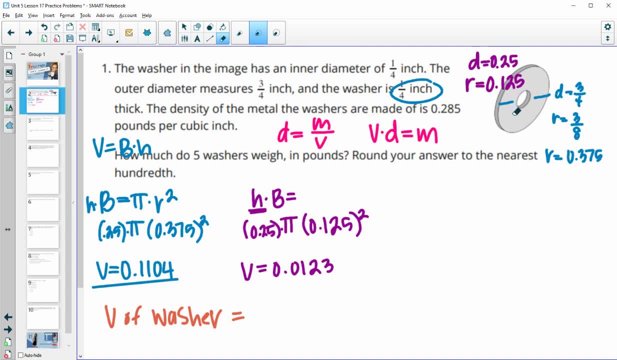 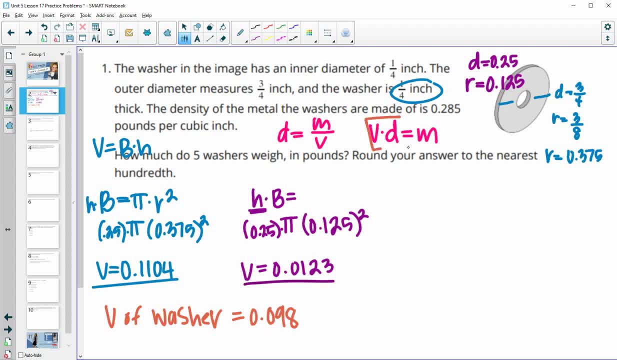 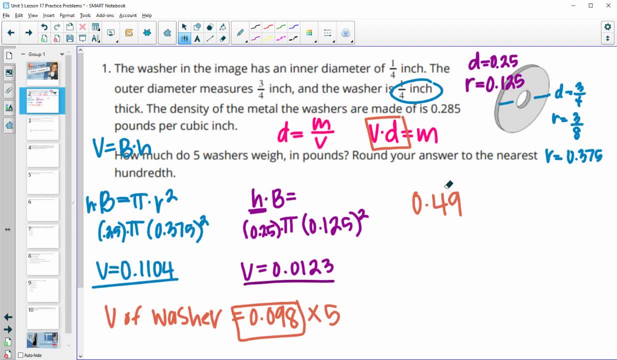 for the, for the volume of five washers, And then we'll take this times the density, and the density per washer is 0.285.. So multiply this by 0.285. And that gives us a mass or a weight of 0.14 grams or pounds, 0.14 pounds. This was in pounds. 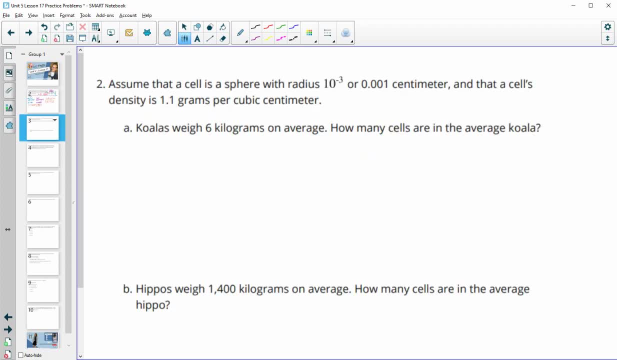 This was in pounds. This was in pounds of this cell, so that we can divide the koalas mass by the cell mass to figure out how many cells there are. And so let's go ahead and figure it out for the cell. So again, volume or density equals mass divided by volume. So we're going to need the volume. We already have the density and that's going to help us get the mass. So again, density times volume. 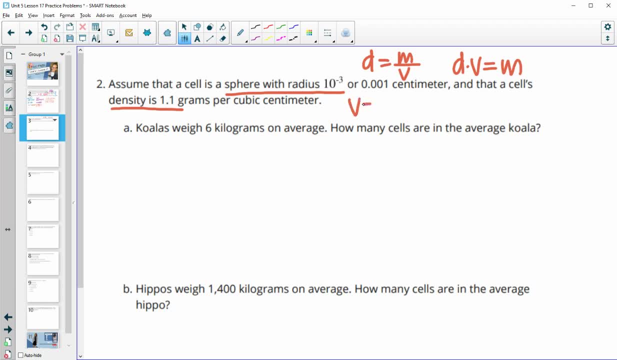 equals the mass. So let's figure out the volume of a cell. Okay, so volume of a sphere is four thirds times pi, times the radius, which is 10, to the negative three, in this case cubed, And so I'm going to leave this. going to be a really small number, So I'm going to leave it in scientific notation. So I'm going to do four thirds times pi And four thirds times pi is 4.1887.. 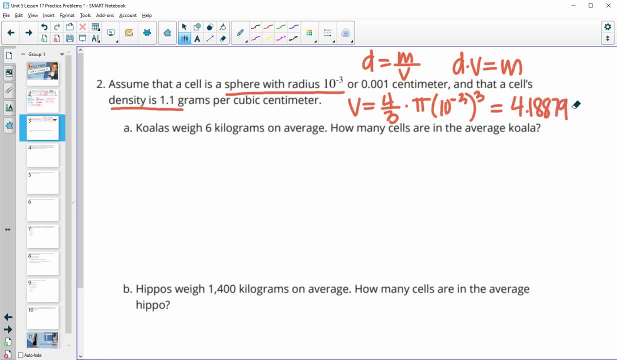 Nine. And then we have this 10 to the negative nine, So 10 to the negative. third to the third would be 10 to the negative ninth. This is the volume of your cell, And then the density of the cell is 1.1 grams per cubic centimeter. So if we multiply this 4.18879, the volume of the cell times its density, that'll give us the mass. 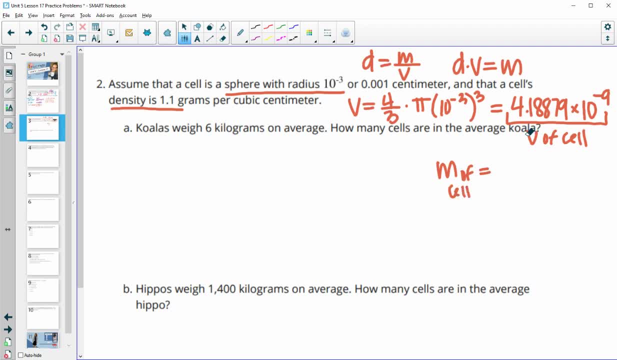 Okay, so the mass of the cell is what we're looking at here. So take this number and multiply it by the 1.1.. So when we multiply 4.18879 times 1.1, we get the mass of the cell to be 4.61 times 10 to the negative nine. So this is the mass of our cell. 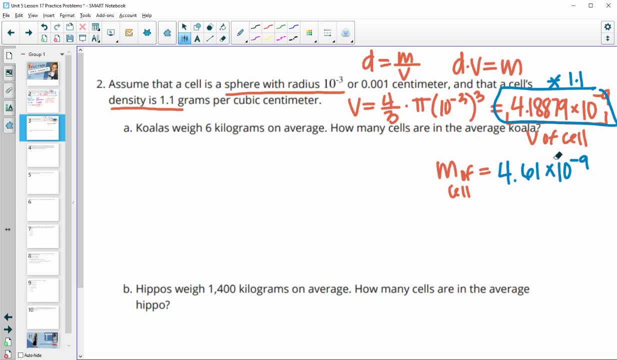 Okay, so now we'll be able to divide these masses by the mass of the cell And that'll tell us how many cells fit into each of these animals. So remember that this one is in grams and here we're in kilograms. So six kilograms in grams would be 6000.. And I'm going to leave it in scientific notation. So this is really six times 10 to the third grams. 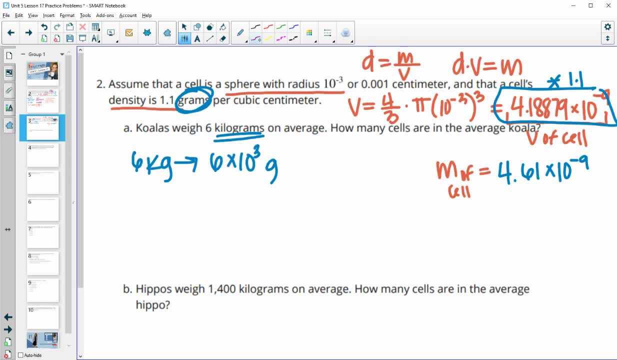 Okay, that's a different way to write it- write 6,000.. So now we'll take and we'll divide this koalas mass by 4.61 times 10 to the negative ninth. So what we're going to do here is we're going to divide the numbers. Okay, so we're going. 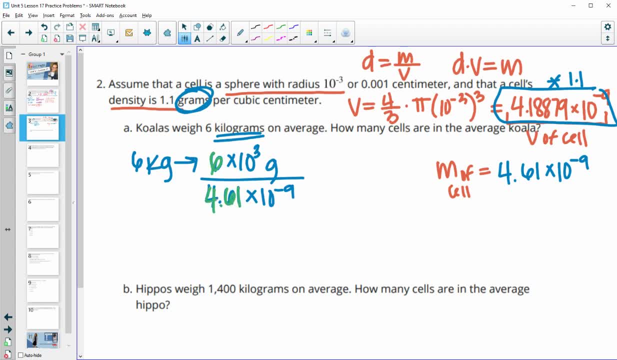 to divide this 6 by 4.61.. So 6 divided by 4.61 is about 1.3.. And then we have 10 to the third, divided by 10 to the ninth, negative nine. And so when you divide powers of the same base, 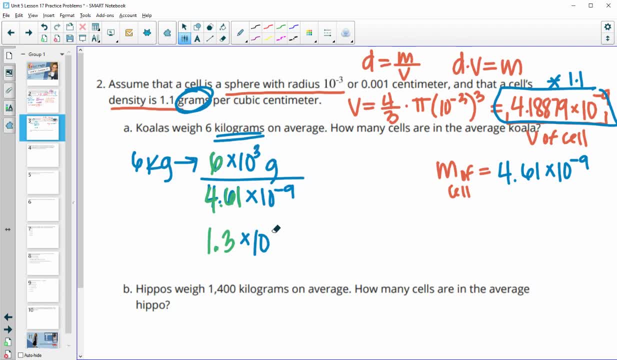 you subtract their exponents, So 3 minus a negative nine is 12.. Okay, so this will really be 1.3 times 10 to the 12. And that's just a really large number. So that's going to move this decimal 12 times. So. 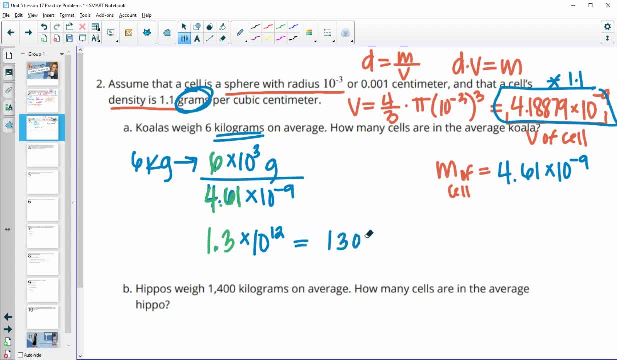 that's really going to be one. And then here's moving it one time: 2, 3,, 4, 5, 6,, 7,, 8,, 9,, 10,, 11, 12.. So this is approximately how many cells this koala has. So this is thousands, millions. 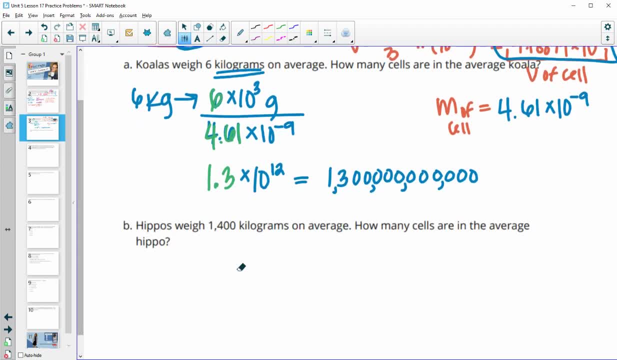 billions, So 1.3 trillion. So then for this one we've got 1,400.. So now this one's already in kilograms. So I'm just going to do this one as 14 times 10 to the second. So I'm just going to take off two of the zeros as 10 to. 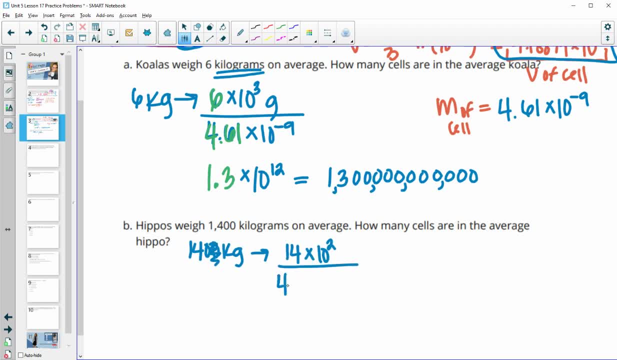 the second, Then divide this by the mass again, which was 4.61 times 10.. Oh sorry, And this is kilograms. So this is going to be. let me redo this. This is not going to be. this is going to be. 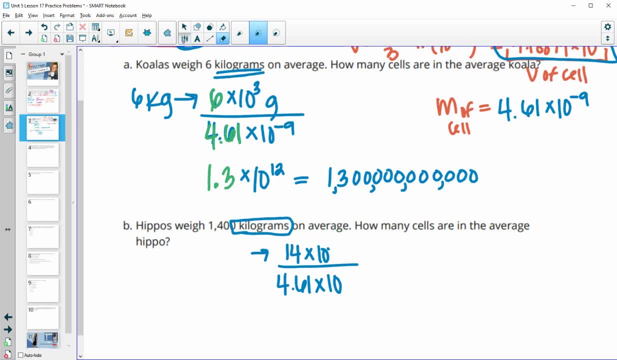 a two, So this is 1,400 kilograms, And so then to turn it into grams, we need to add three more zeros, So then that's 1.4 million grams. So now I'm just going to take off all these zeros, So I'm 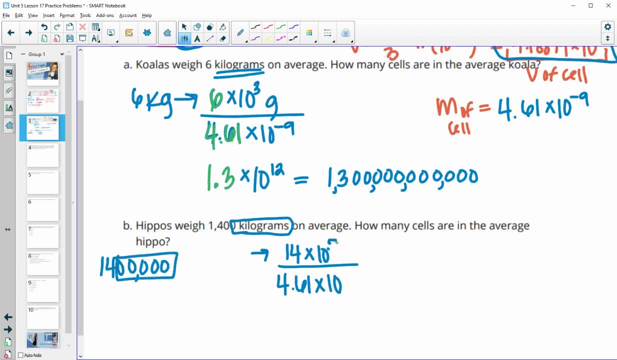 just going to leave it as 14 times 10 to the fifth, just because it's such a big number. So now we're going to do the same thing here. We're going to do the same thing here. We're going to do the. 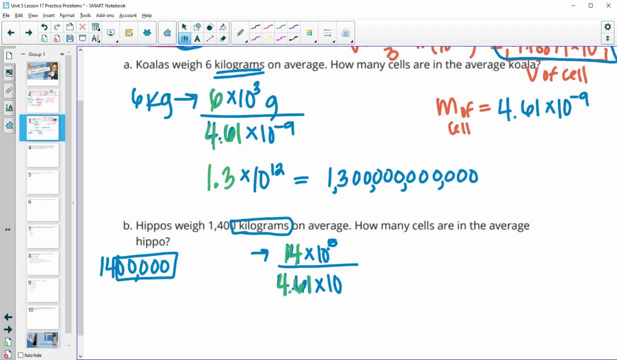 14 by the 4.61.. So 14 divided by 4.61 is about 3.03.. And then when we do 10 to the fifth, divided by 10 to the negative ninth, So five minus negative nine gives you 14.. So this one will be. 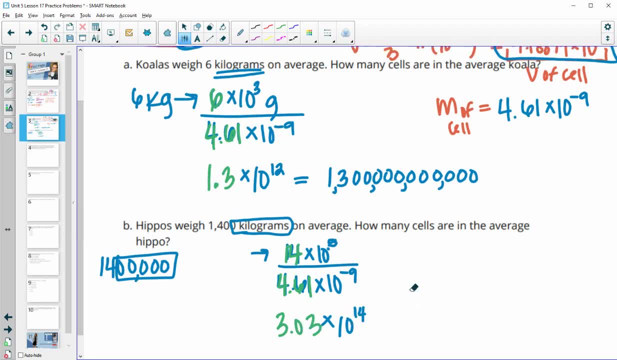 3.03.. times 10 to the 14th cells. And then again you could write it out. So then we'll move the decimal place. So here's moving at 1,, 2,, 3,, 4,, 5,, 6,, 7,, 8,, 9,, 10,, 11,, 12,, 13,, 14 times. So then this is how. 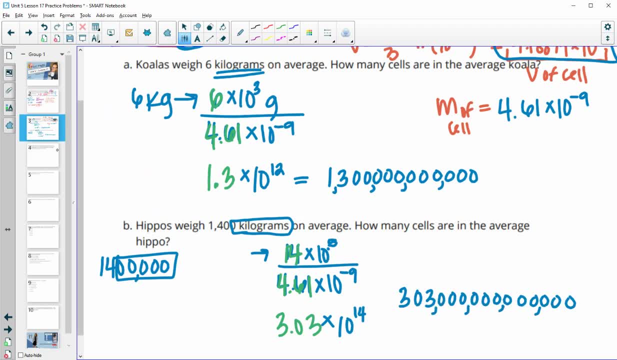 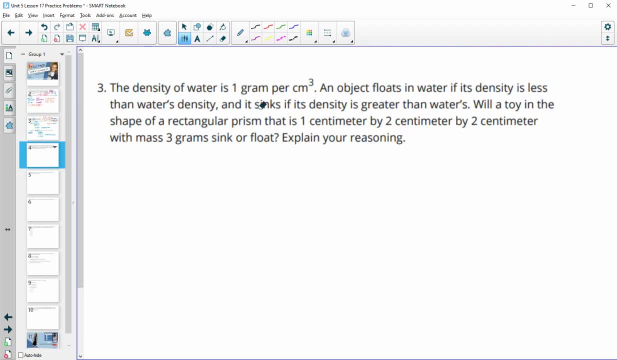 many cells would fit in a HIPPO, or how many cells there are in a HIPPO. Number three, the density of water is one gram per cubic centimeter. An object floats in the water, So this is going to be in the water if its density is less than the water's density, And then it sinks if it's greater. 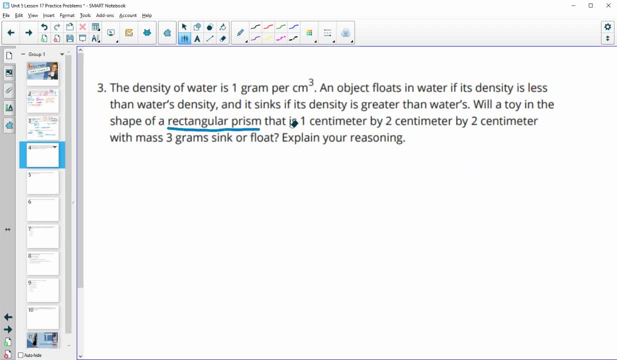 So will it toy in the shape of a rectangular prism. That's one by two by two, with a mass of three gram sinker float. So we need to figure out its density, So we're going to need its volume, And so here's just a quick picture of it. And so it's going to be like a two by two by one. So you just 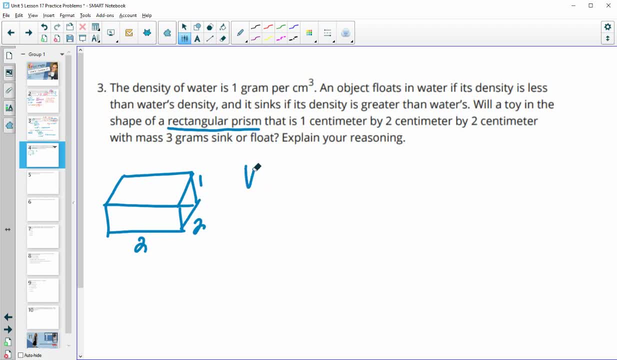 multiply all those together for a rectangular pyramid, A rectangular prism's volume. So two times two is four, times one is four. So this one has a volume of four centimeters cubed. And remember it told us its mass is three. So then the density is equal to the mass divided by the volume, And this is a density of 0.75,. 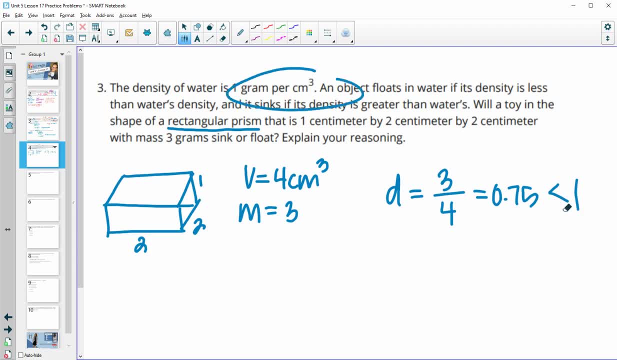 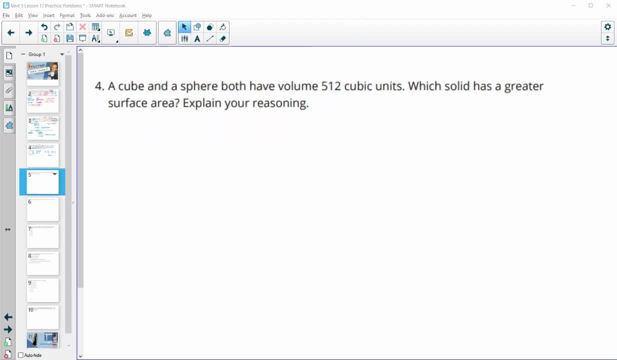 which is less than water's density of one. So this one's going to float. Number four: a cube and a sphere. both have volume of 512 cubic units, Which one has a greater surface area. So let's go ahead and take the cube, figure out one of its lengths and then figure out its. 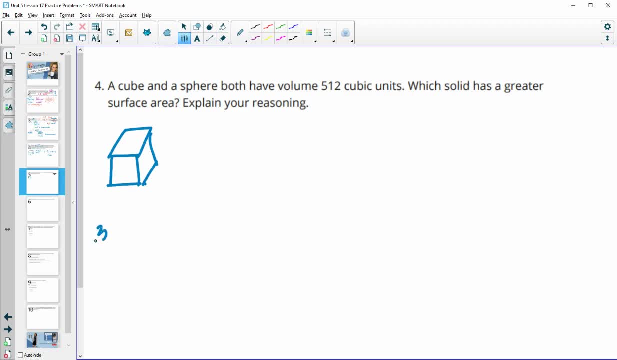 surface area. So for the cube to get the length, you can just cube root the 512, since they're all the same. So the cube root of 512 is eight. So each of these lengths are going to have a volume of 512. 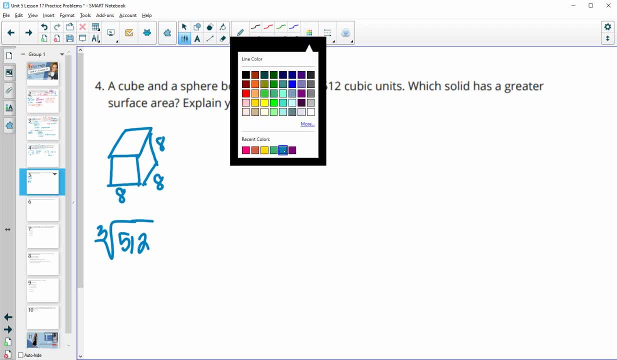 Each of these lengths on the cube is going to be eight. So then, to find the surface area, you would just take: eight times eight gives you that one surface's area is 64 square units, And then a cube has six surfaces, So the cube's surface area is going to be 64 times six. 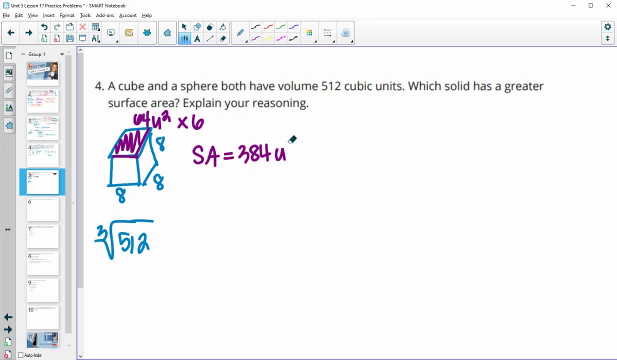 which is 384 units squared. So then we'll want to do a similar thing for the sphere. So now the volume formula for a sphere is a little bit more complicated. So it's four thirds times pi, times the radius cubed. So we know that the volume is 512.. So we're just going. 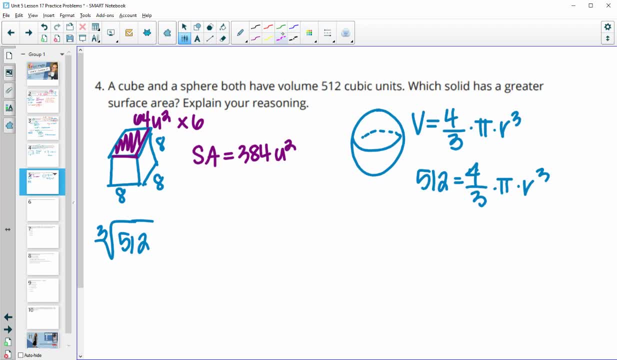 to need to work this formula backwards. So we're going to multiply both sides by three fourths to cancel out that four thirds, So three fourths of 512.. Is 384.. So we get: 384 equals pi times our radius cubed. So we'll divide by pi. 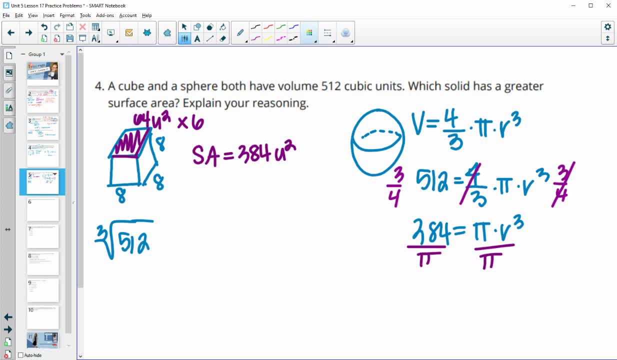 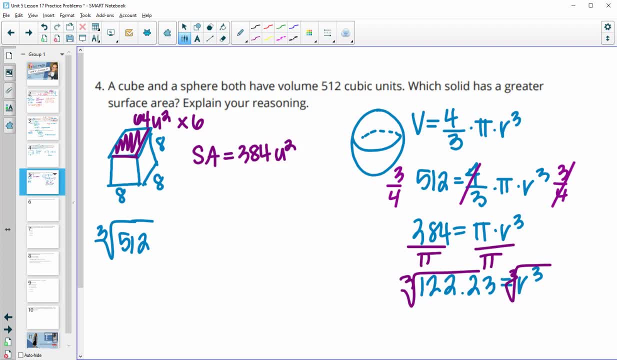 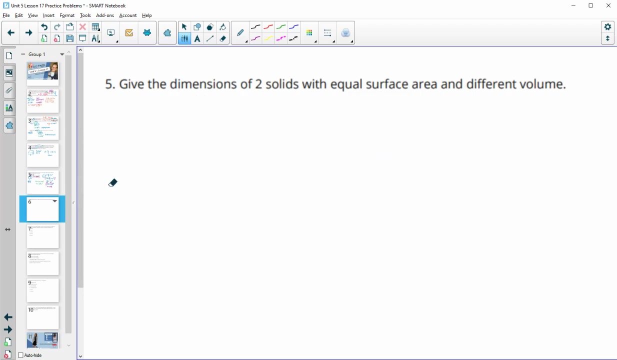 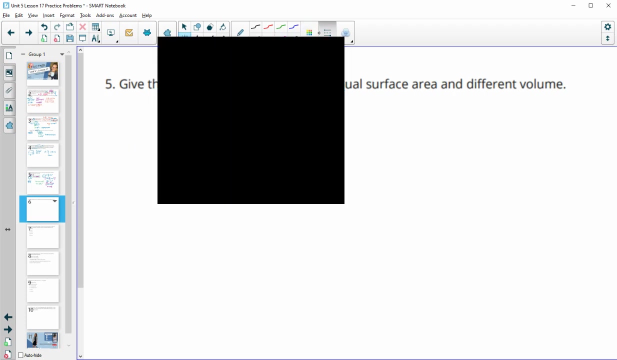 So we're going to do 384 divided by pi, And when we do 384 divided by pi, we get about 122.23.. So we're going to do 384 divided by pi, And when we do 384 divided by pi, we get about 122.23.. 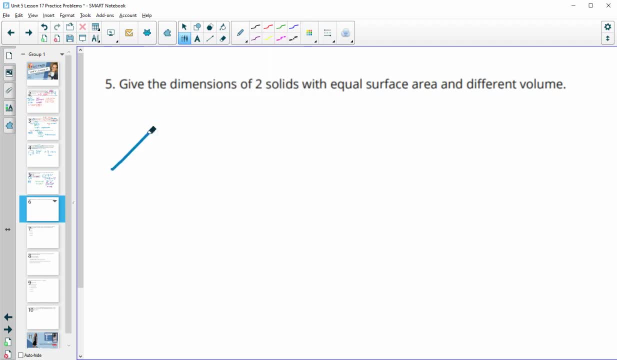 So we're going to do 384 divided by pi, And when we do 384 divided by pi we get about 122.23.. gonna do two rectangular prisms, so I'm just gonna make up some dimensions here. so I'm gonna start with a base of 10 by 2 and then I'll do a height of 3. so then 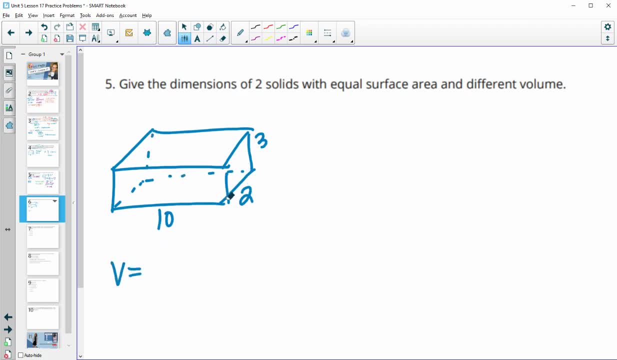 this will give me a volume of 10 times 2 is 20 times 3 is 60 units cubed. and then, for the surface area, we're gonna have two surfaces that are this size, which are 10 by 3, so two 30s. so I'm gonna have 30 plus 30, and then I'm gonna have two. 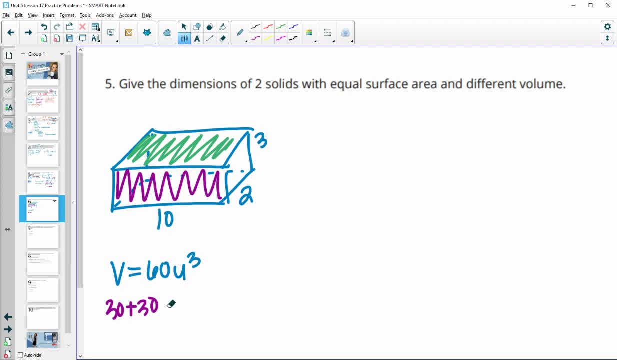 of these surfaces, top and bottom, that are 10 by 2, so those are each 20. and then I'm going to have two of these surfaces here which are 2 by 3, so those are each 6, and so this is gonna give me a total surface area of 112 units squared. so 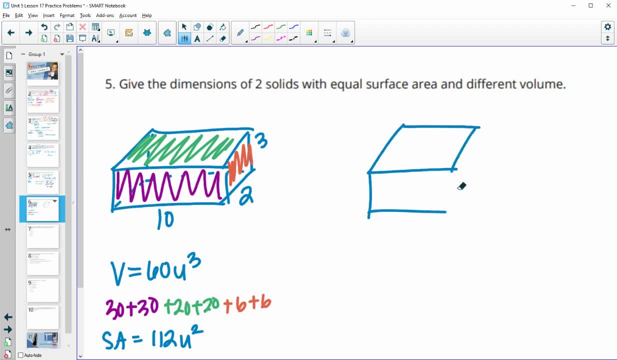 then I just need to create another one that has the same volume but has a different surface area. so I'm gonna leave the height at 3, so I know I still need my base to be 20, so I'm just gonna change the dimensions to 4 by 5, so 4. 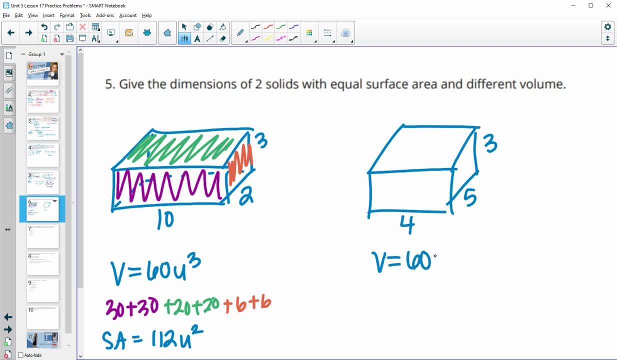 times 5 times 3 still gives me a volume of 60 units cubed. But now the surface area will change. So I've got two of these surfaces which are four by three, So that's 12 plus 12.. Then we have this surface which is five. 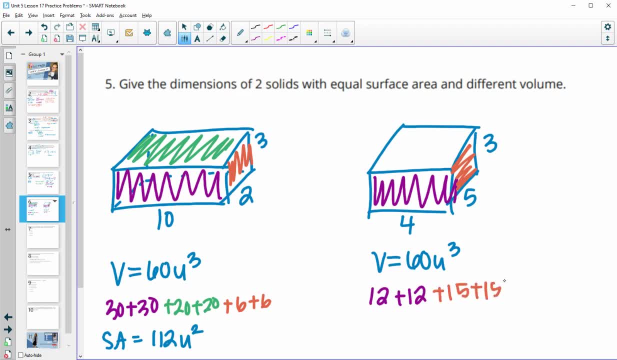 by three, So we're going to have two of those, So two 15s, And then our base top and bottom, are going to be four by five, So those are going to be 20s, And so if I add all of those up, 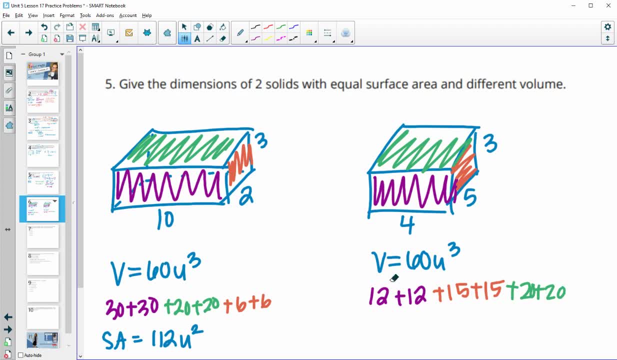 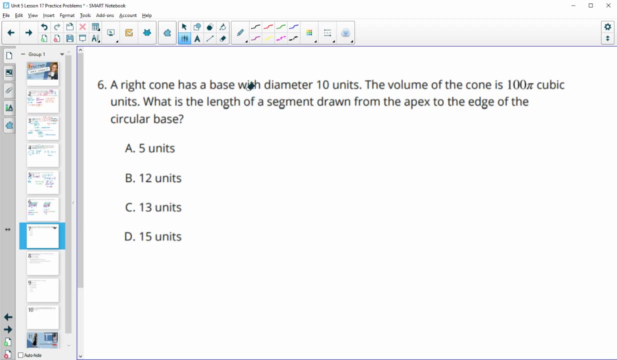 I will end up with a surface area here of 94.. Number six: a right cone with a base that has a diameter of 10 units, And then the volume of the cone is 100 pi cubic units. What's the length of the segment drawn from the apex to the edge of the? 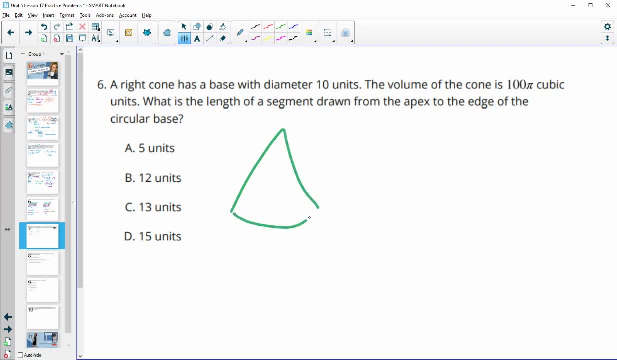 circular base. So let's get a picture drawn of this. So we know that this radius is 5, since the diameter was 10.. So we can figure out: the base area here is going to be pi times that radius squared and they're leaving it in terms of pi, So I'm just going to put this base area as 25 pi. 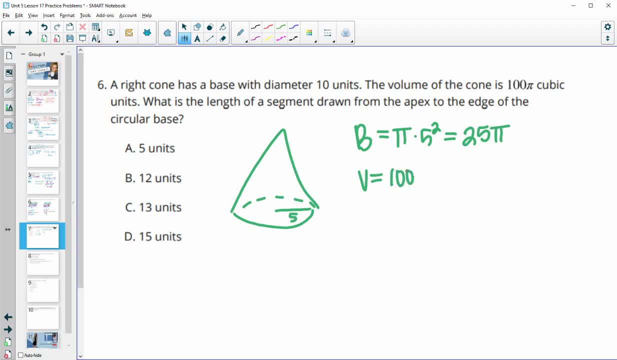 Then they're telling us that the volume is equal to 100 pi. And remember, for a cone, the volume is area of the base times the height divided by 3.. So let's multiply by 3 first to get 300. pi will equal our base area times our height. 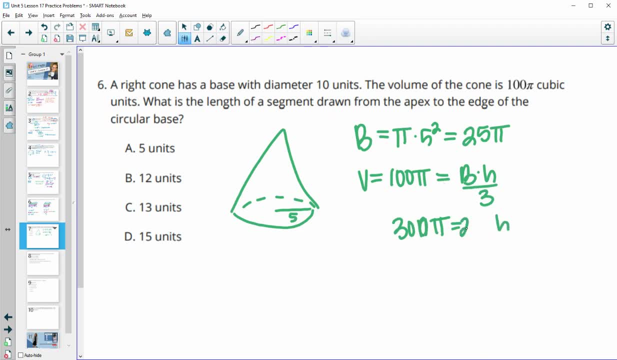 And then we know the base area is 25 pi. So we can just divide by 25 pi to figure out the actual height here. And so 300 divided by 25 gives us 12, since those pi's cancel out, So our height here is 12.. Now they wanted the. 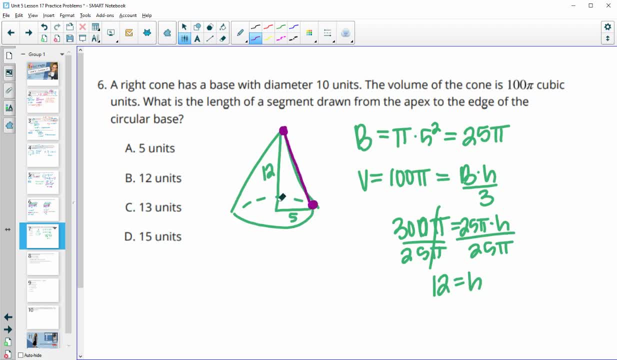 length of the segment that runs from the apex down the side. So now we're going to have to do the Pythagorean theorem here to figure out this length. So the hypotenuse squared equals the two legs squared and added together. So then this is going to be 144 plus 25, which is 169. 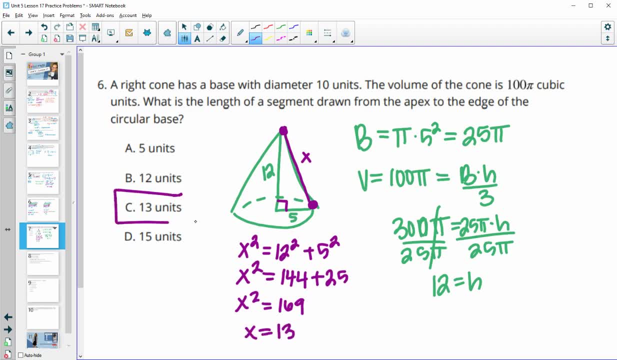 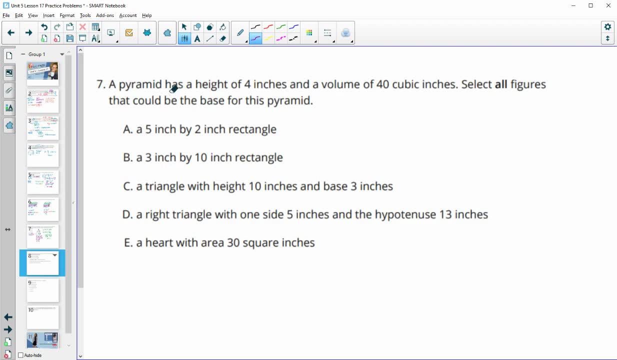 And then we'll square root that and we get 13.. All right, number seven: a pyramid has a height of 14. And a volume of 40.. Select all figures that could be the base. So remember, a pyramid has a volume. 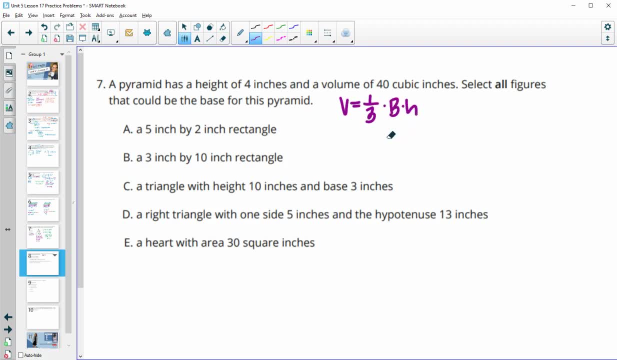 of one third times the area of the base, times the height. So I like to work this backwards. So we're at: 40 equals one third times the area of the base, times four, which is our height. So let's multiply both sides by three to get rid of that one third, And then let's divide by four So we have a volume. 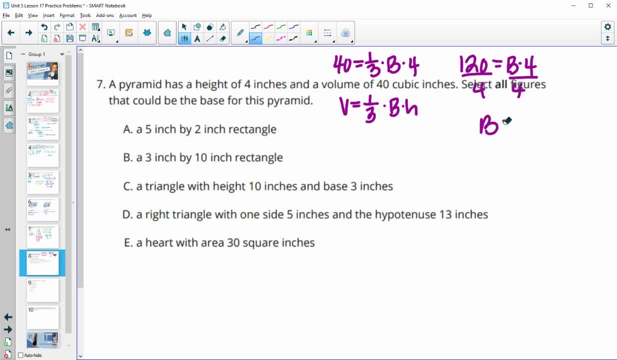 of 30 capital pieces And let's see if our spice needs 30 and we're at 40. Let's probably fit together this whole thing in a choice, All right. so 10 times four divided by four, to figure out that the base area needs to be 30. So if our base area is 30, that will give us a volume of 40 cubic units. 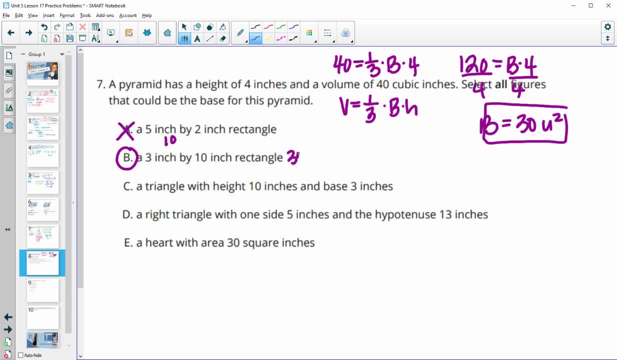 So this rectangle five times two is 10.. So this is not going to work. Three times 10 is 30. So this one would give us 30 units squared for the base area by 2.. So 10 times 3 is 30, divided by 2 is 15.. So this one wouldn't A right triangle with one side. 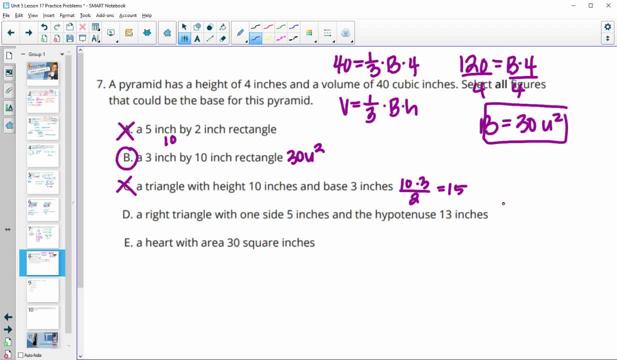 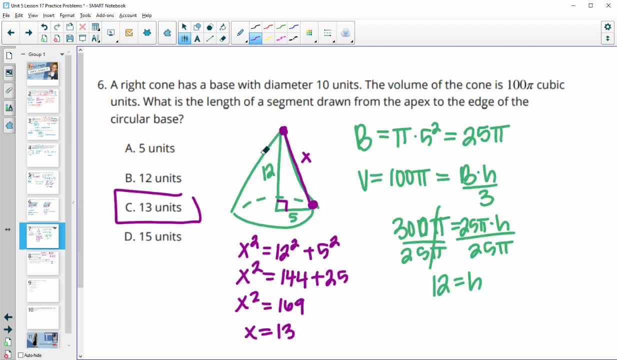 is 5 inches and the hypotenuse is 13.. Well, this is the same triangle we just did on the last problem with 5 and 13 here. So, if you remember, the other side was 12.. So then we know that that's. 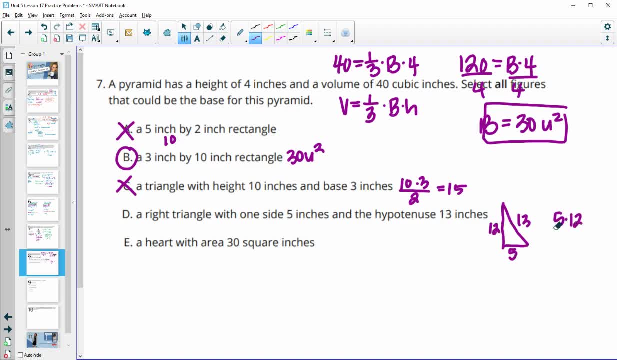 12.. So 5 times 12 divided by 2, for the area. Well, 5 times 2 is 60, divided by 2 is 30. So this one will be good, And then a heart shaped, or a heart that has an area of 30. That'll be good. 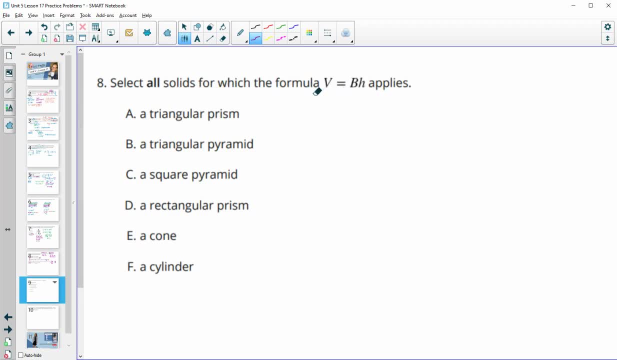 Number 8, select all solids where the formula area of the base times the height applies for the volume. So a prism, yes. A prism, yes. A pyramid: no, because this will be divided by 3 since it goes to a point. So no for the pyramid. 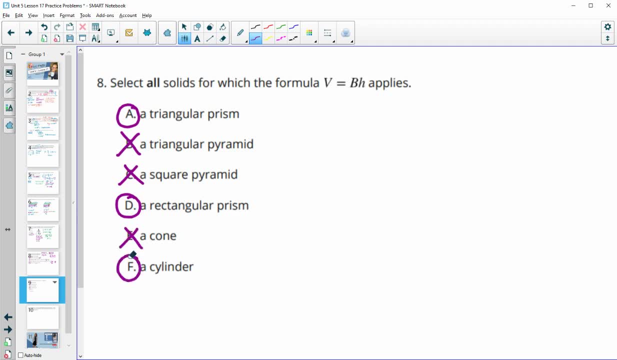 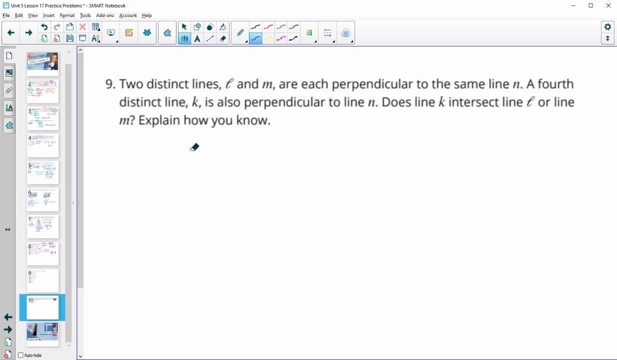 yes for the prism, no for the cone. yes for the cylinder. Number 9,. two distinct lines, L and M, are each perpendicular to the same line N. So if I draw N, okay, line L needs to be perpendicular to it and line M needs to be perpendicular. 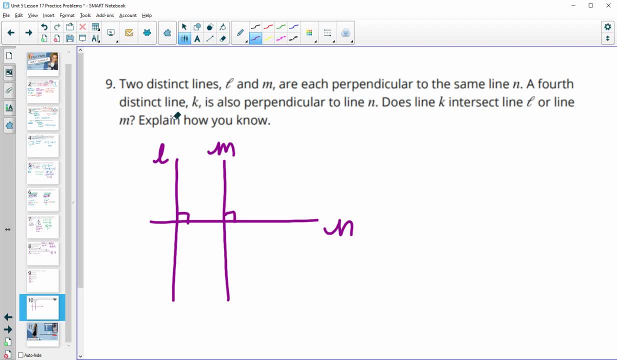 So if I draw N, okay, line L needs to be perpendicular to it and line M needs to be perpendicular to it. A fourth distinct line- distinct, just meaning different, so not on any of these- Line K is also perpendicular to N. Does K intersect these other two lines and explain how you know And the answer?